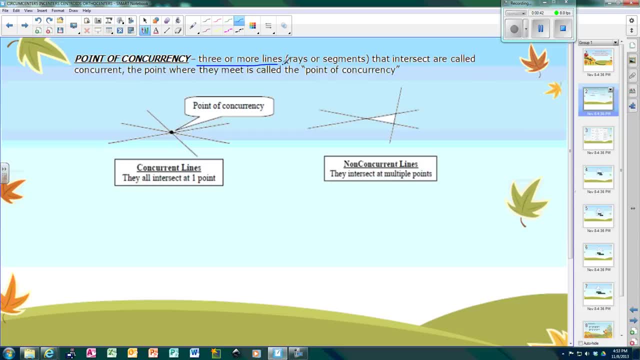 concurrency. So that's when you have three or more lines that intersect, They're called concurrent lines, And where they intersect is called the point of concurrency. So, for example, we've got this line here, So we've got this line that goes through here, And then we have this line that goes. 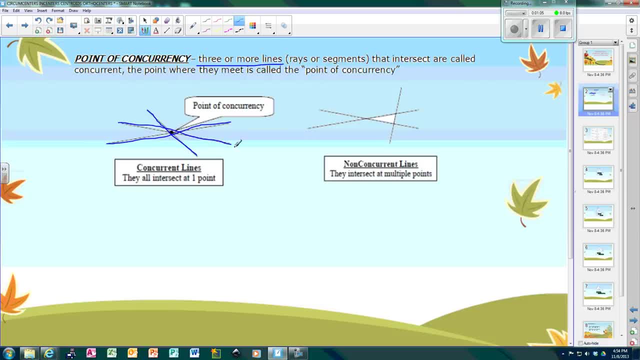 through here And then we have this line that goes through here. So they all intersect at one point and it's called the point of concurrency, Kind of like when there's a bunch of streets that intersect. So it's called the point of concurrency, where they intersect. These would be considered. 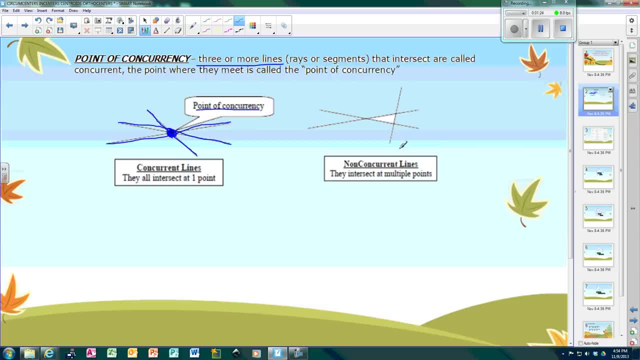 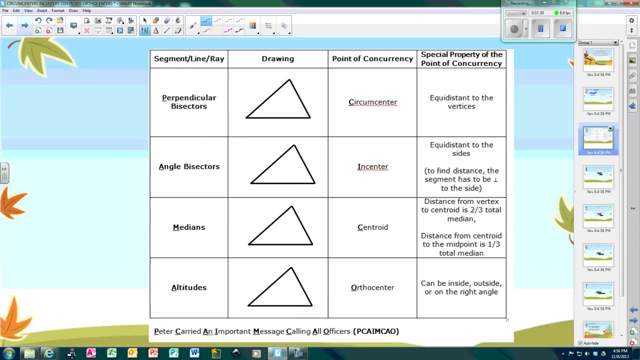 non-concurrent lines, because you only have two intersecting lines, So it's called the point of intersecting at a time, Okay, Okay, So here we've got our non-concurrent lines and our concurrent lines. So let's hide this, All right. So let's talk about what happens here, Okay, So remember, we had 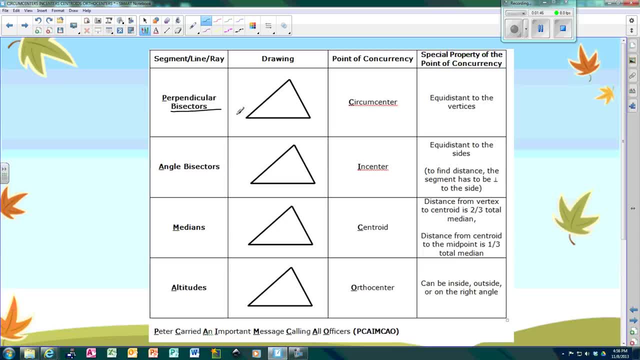 our perpendicular bisectors. The word bisector tells me that I need to find the midpoint of each side. So since my triangle has three sides, then I'm going to have three midpoints. So I'm going to have three midpoints here And I'm just kind of eyeballing them, And a midpoint here So they may. 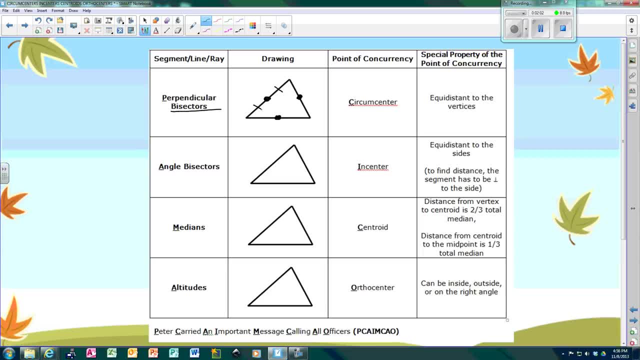 not work out to be perfect, but they'll be close, So make sure you put the marks on here. I'm going to put two here, I'm going to put one on this one and three on this one. Okay, So that tells me this. 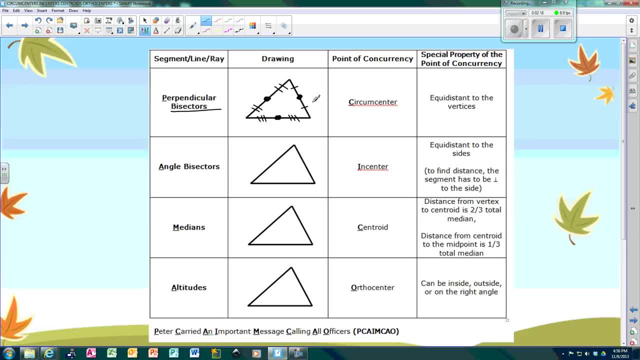 is the midpoint because those two are congruent. This is the midpoint because those are, And this is the midpoint because those two are Okay. So now, perpendicular It means it has to be right angle through that point. So I'm going to go to the point and I'm going to just draw a ray. 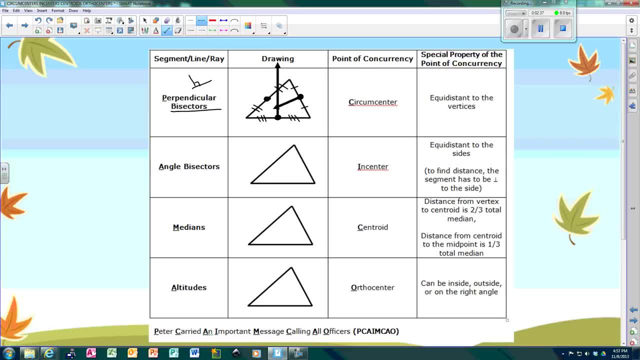 straight up. And the same thing here. I'm just going to just kind of eyeballing it, Going to the point and straight up. So now I've got three perpendicular bisectors, And I know they're bisectors because I created their midpoints. And now I know they're perpendicular because I am. 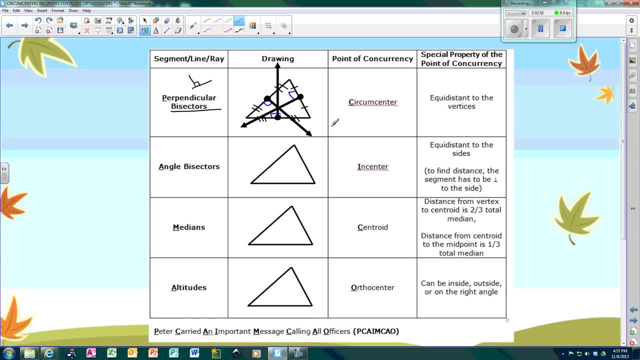 right angle marks. Do not forget those marks. Now there's something that's really really cool about the perpendicular bisectors, And we'll go into this later, But if you go to their point right here where they intersect, So I'm going to put me a point where they all intersect. 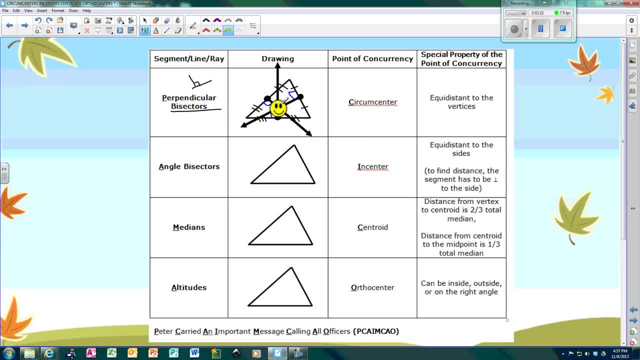 Okay, They all intersect right there. So that point right there where they all intersect, is the point of congruence. And I'm going to go to the point where they all intersect And I'm going to put me a point where they all intersect. So that point right there where they all intersect, is the 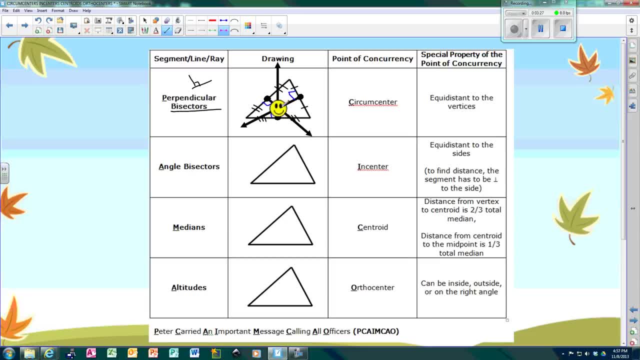 point of concurrency. Okay. So now what's really cool about them is if I go to the point and I draw a line That is just way too big. So if I go to that point where they all intersect And if I draw a, 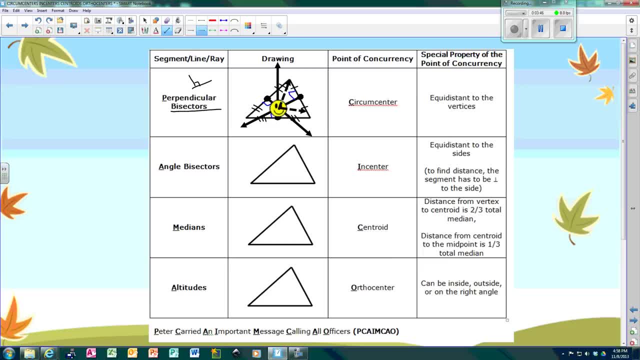 line to each corner. So we have a bunch of different lines. It's a little bit confusing. Those three lines that I just drew are all the same, So I'm going to go to the point where they all intersect And I'm going to say I want it to be at the same length. So there is a whole lot of stuff that is. 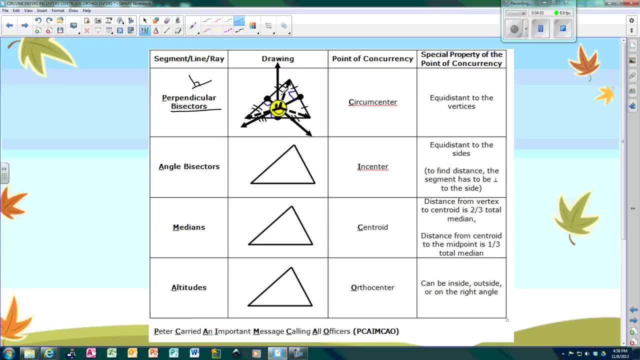 congruent here, Because we've got all these pieces that are congruent and now these little lines right here are all congruent. Okay, So all those arrows are congruent. So we need to remember they are equidistant, which means same distance from the vertices. So from here to each corner. 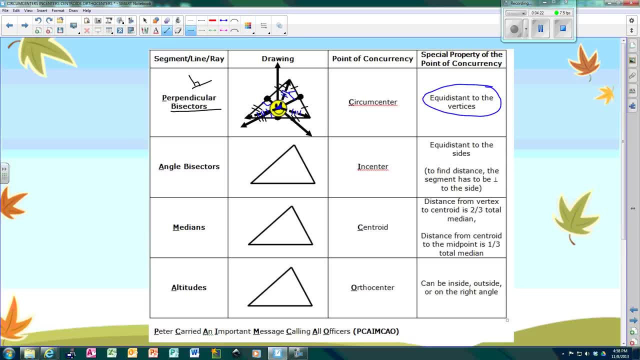 And we will get more into that later. Okay, Now we have angle bisectors, So you go to their point. They all intersect. That is to contain the growing Bernie, but many of the lines in the point are congruent. They all intersect. They all intersect, That is to contain the growing Bernie, but many of the lines in the experts even you can see that all are grown together. Here we can see each orange line is congruent. This is going to tag along the point. 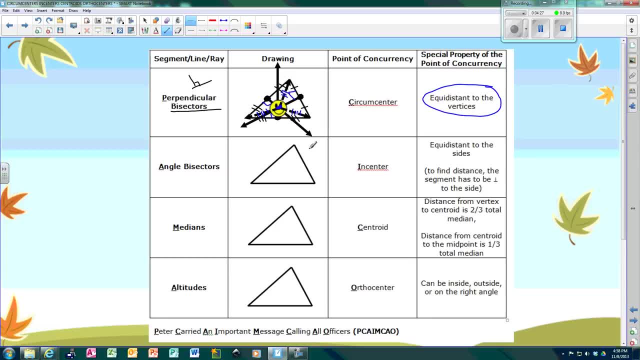 so you go to the angle. can i not just get a straight line? so i'm going to just eyeball it close enough. come here, eyeball it. go here, eyeball it, all right. so now i have my point of concurrency. so right here, where they all intersect, okay, my thing is definitely not functioning today. 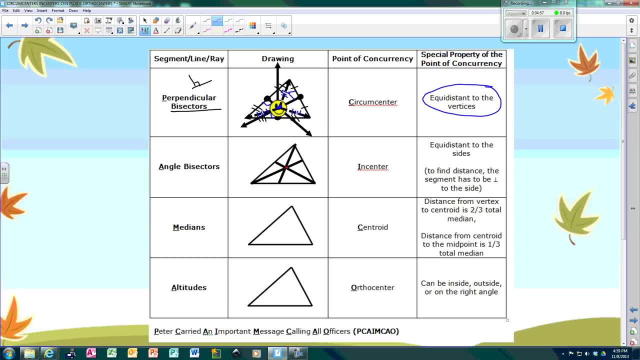 so where they all intersect, this point right here. this is called your end center. okay, it is equidistant to the sides. so to find the distance, the segment has to be perpendicular to the side, and we'll talk about that more later. so remember, i told you they all had something special well. 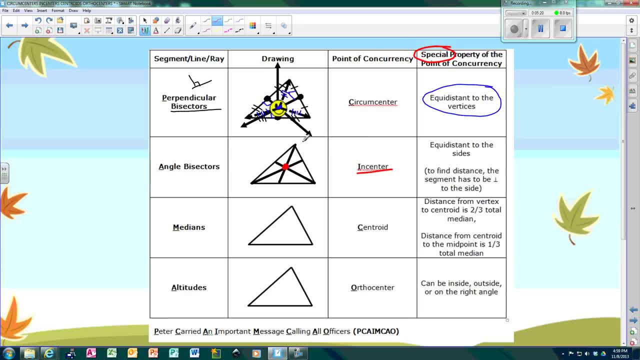 that's what's special about an angle bisector. all right, the next thing we have is our medians. okay, the medians. remember we need a midpoint first. so i'm going to find the midpoint of each piece again. so again, we're just going to kind of eyeball it so that piece is equal to that piece, because i 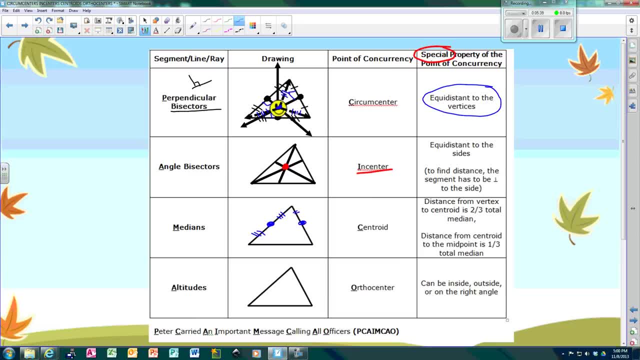 created a midpoint. this piece is equal to this piece and this piece is equal to this piece. and now the medians. if you remember from earlier, you start at your corner and you just connect to the to the midpoint. go to this corner. connect to the midpoint. go to this corner, connect to the midpoint. 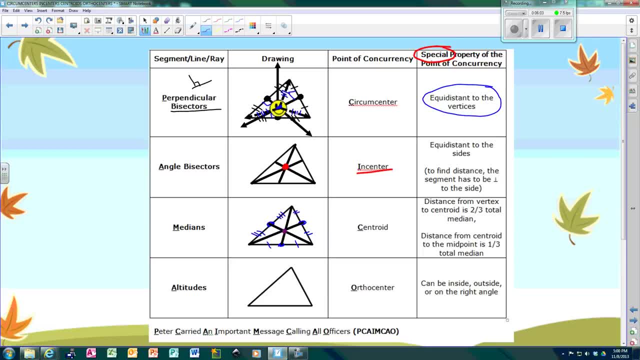 and guess what, where they all intersect. that's their point of concurrency and it's called the centroid. and what's cool about the centroid is that this top distance right here, the one that starts at the corner and goes down, is two-thirds of the whole thing. so if you thought about it, if 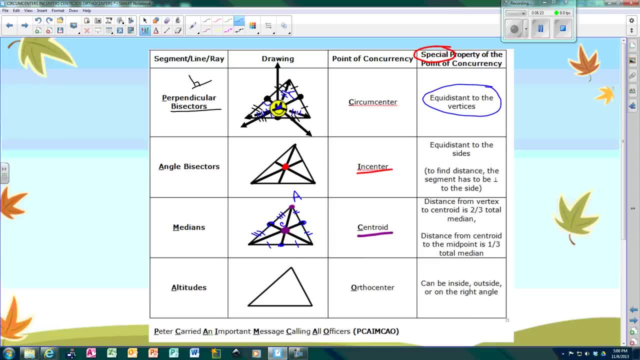 i called this a and i'm going to call this centroid c, i'm going to call the midpoint m. then i would say that a c is two-thirds of the whole thing. a m, which means this piece down here would be one-third all right. and then our next one is an. 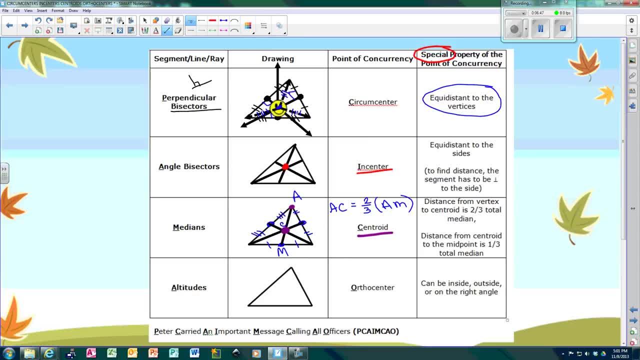 altitude. this one is, i think, pretty easy, because you just go to your corner and drop a line straight down. so go to the corner and straight down. go to the corner straight down. it doesn't have to be at the midpoint or anything, all you do is you go to the corner and straight down and it has to be perpendicular. so you have. 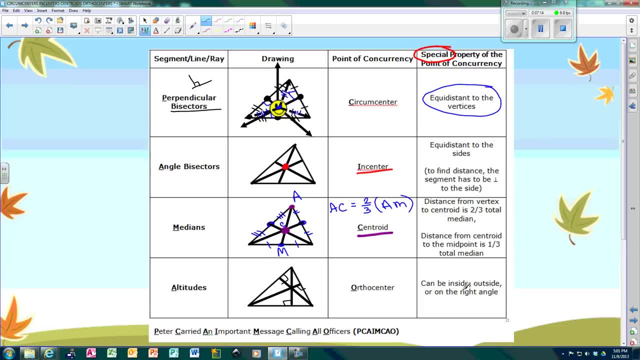 to make sure that you put the mark that says that it's perpendicular. and the cool thing about it is it can be inside or outside, or it might even be on the right triangle. so now you have to remember, remember which one of these points goes with which set of lines. so one way you 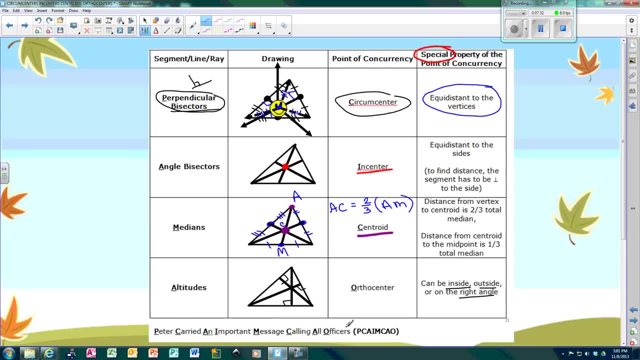 can remember is the sentence Peter carried, an important message calling all officers, or the way I like to do it, I like to use this one. I like to say: pretty cats are inside, mean cats are outside, because that means perpendicular bisectors go with the circumcenter angle bisectors go with the in-center. 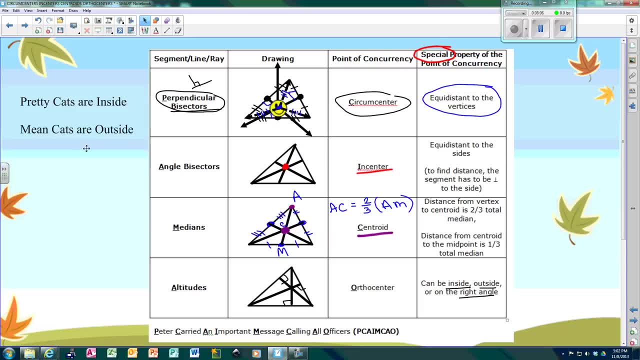 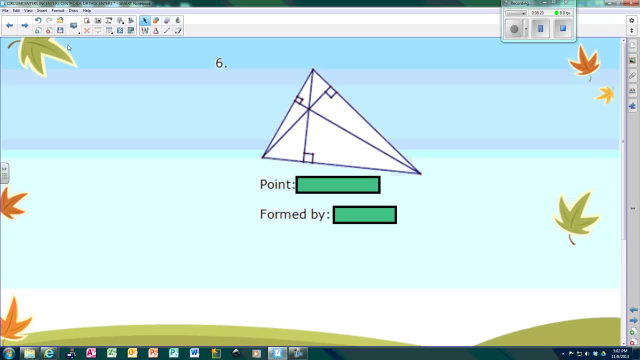 medians. go with the centroid altitudes, go with the orthocenter. to me, this one is easier than this one. you may like this one. you may be even creative enough to come up with your own, so let me know if you do. all right, so now let's talk about this. we're going to decide based on these markings. 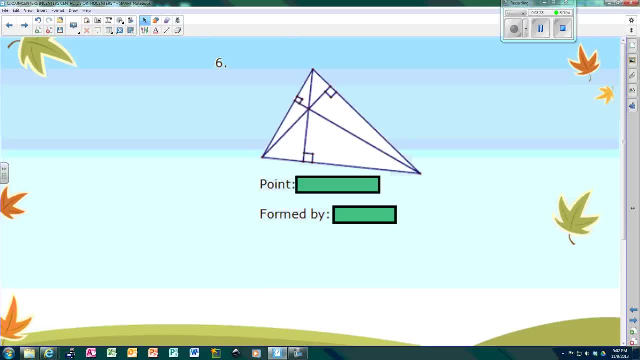 which lines are they? so we are starting at our corners and we're perpendicular. so that means it has to be an altitude, and if pretty cats are inside and mean cats are outside, so I'm thinking let's go back here. I'm going to clone this, actually, I'm just 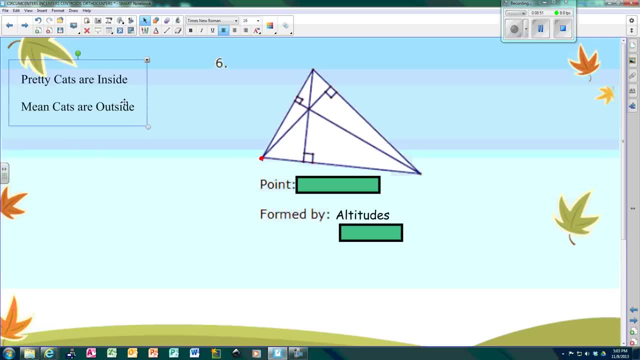 gonna copy it and then I'm gonna paste it on this side. so I have it. so I'm thinking, in this particular sentence, pretty cats are inside, so these are my bisectors. perpendicular bisector and angle bisectors mean cats are outside, so altitudes, go with the one that starts with an O, which is the orthocenter. ok now 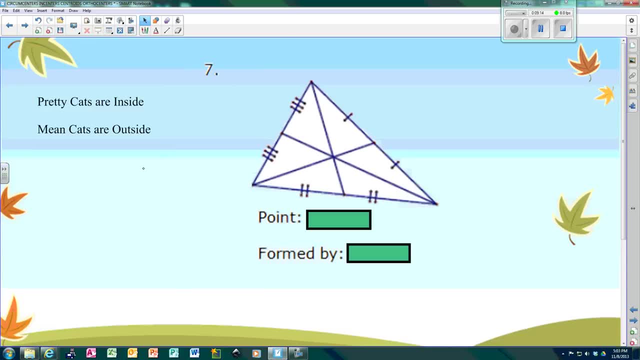 let's do it again over here. so we have our reminder. this time. I look and I see, well I have, this piece is equal to this piece, so this has to be a midpoint. that has to be a midpoint, that has to be a midpoint. well, I'm going to my corners, so the corner to 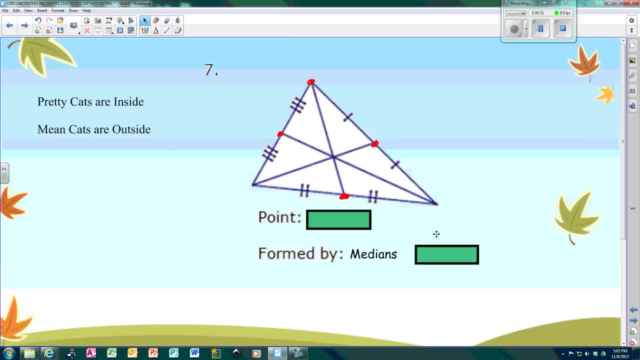 the midpoint is a median, so median is mean, so it has to be the one that starts with a C. so I always think median, middle center, centroid, all those things kind of mean the same thing. okay, now this one. I just have congruent angles, okay that's.